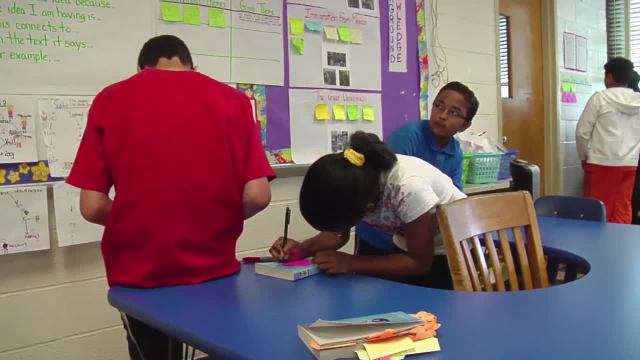 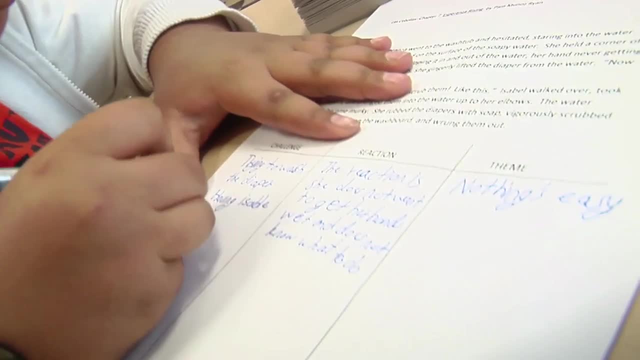 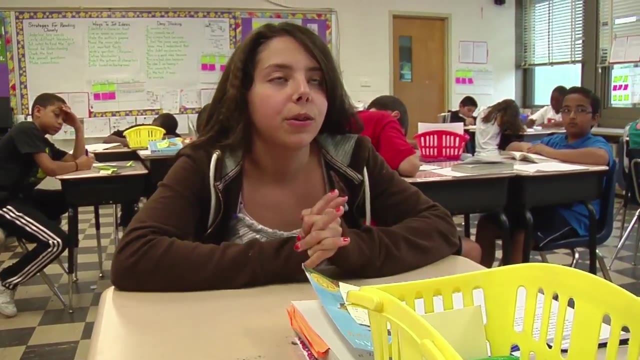 And so having them physically writing down those details, find proof, find evidence over time was what really got them to zoom in on. what was important, Emily, what made your ideas change about what the theme was of the book, How in the beginning, how all those challenges and everything happened to her? 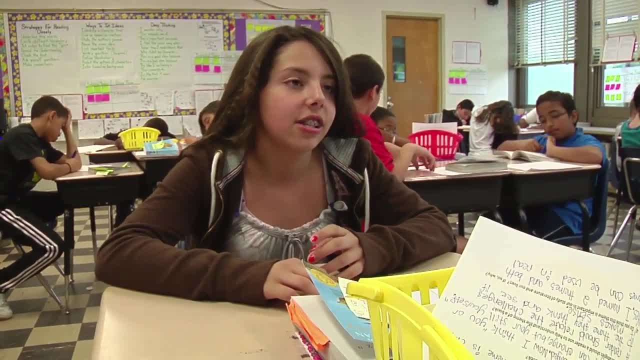 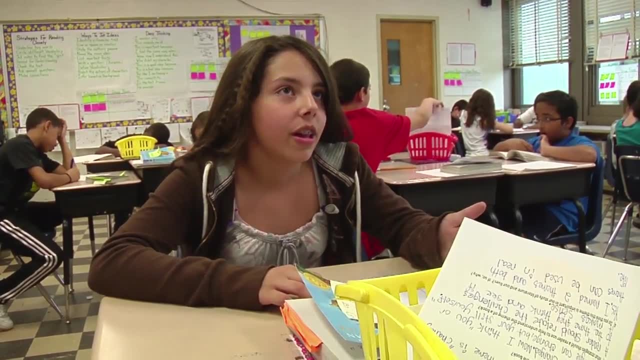 But now I think that since she's still now, she went from rich to poor. she's changed a lot, but she's still herself, Like. she's still like. I want, I don't want to work, I don't want to do anything like this. 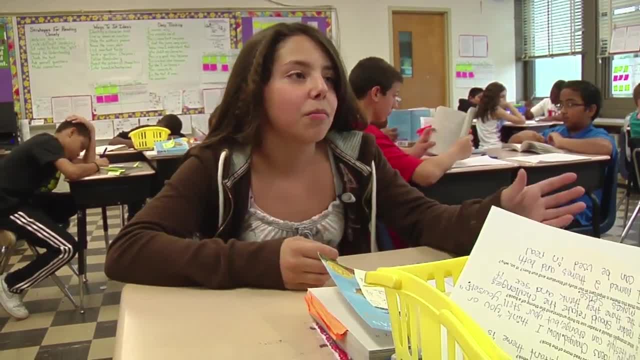 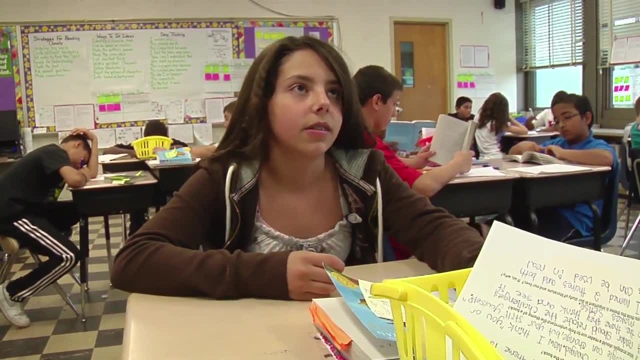 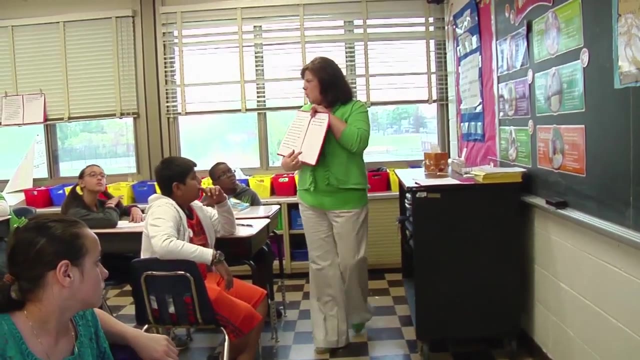 So she's still her and she's not rich, But she's still herself, So she's not fully changing based on what happened to her Interesting. In recent teaching we've been going from a big idea to a smaller idea of finding specific details. 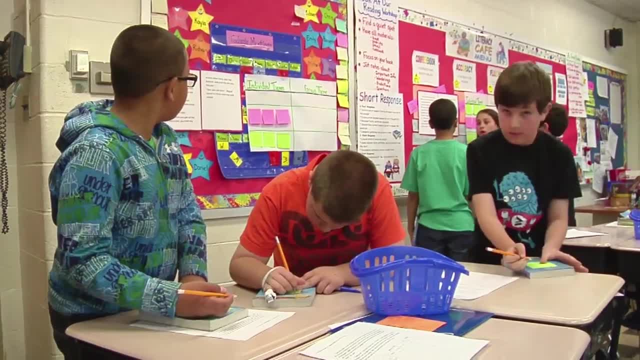 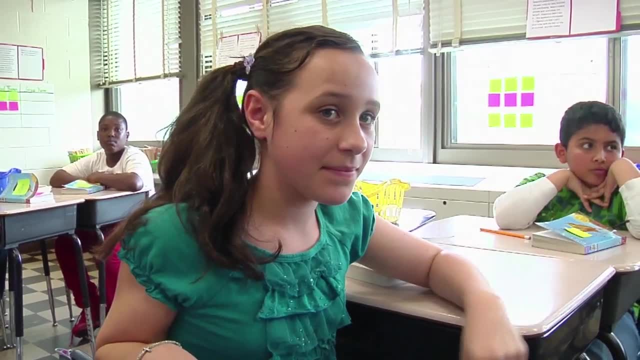 And I wanted my students to have the experience of taking those small pieces- and thinking more analytically- into a larger literary element, a bigger picture, seeing the bigger picture. So let me show you what I mean when I say that we're going to be relating some chapters. 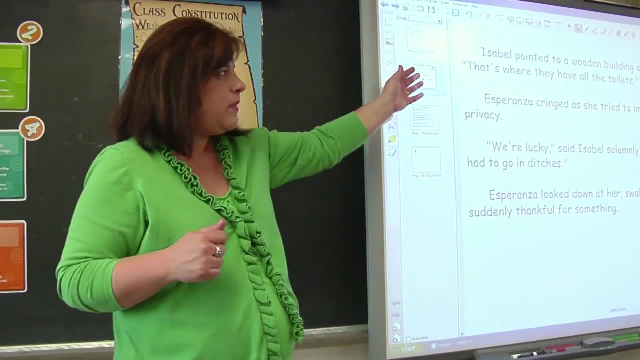 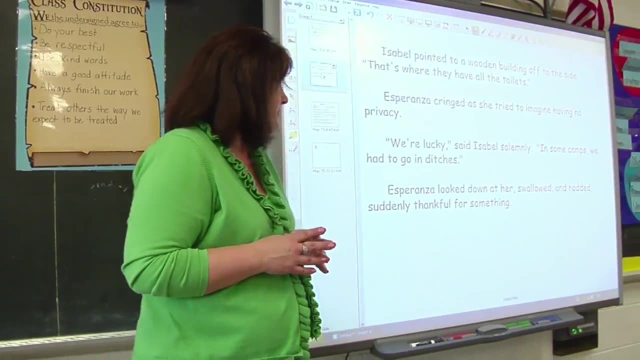 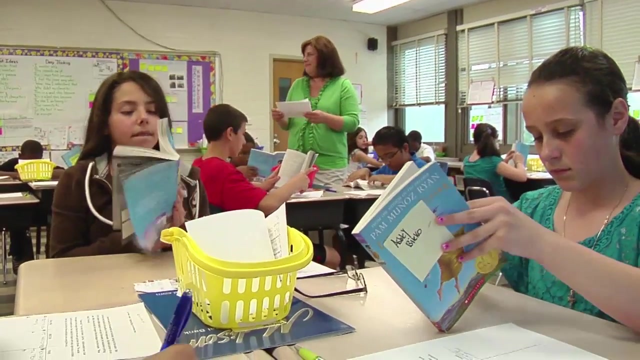 And I want you to take a moment to think about what were our main challenges to a theme. okay, Isabel pointed to a wooden building off to the side. That's where they have all the toilets. Esperanza cringed as she tried to imagine having no privacy. 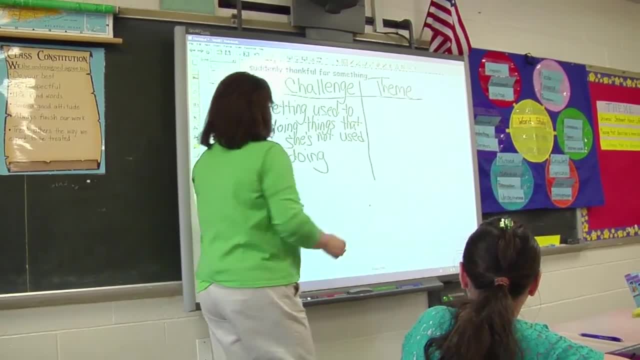 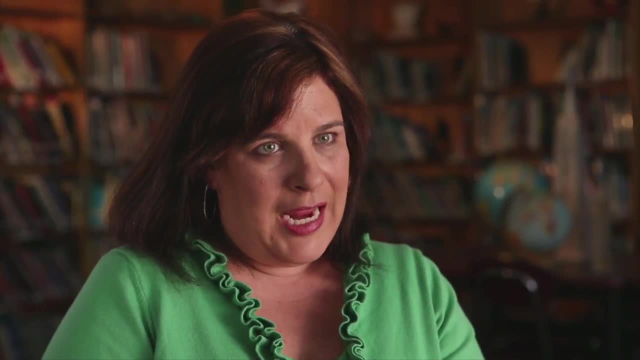 Well, they started out reading the entire chapter on their own. Then we revisit the chapter a second time and do more of a comprehension type activity. So it kind of builds over time to get to the point that you saw here, saw today. so now i'm going to give all of you a piece of text evidence to work on with your group. 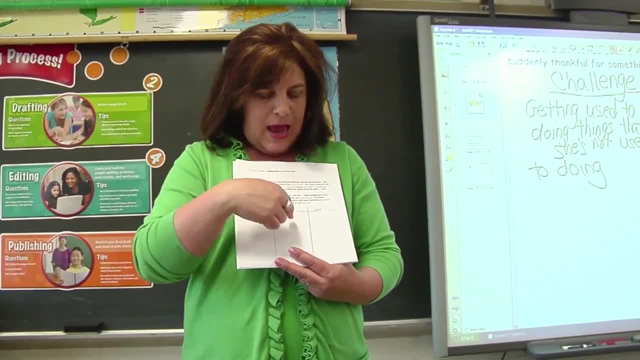 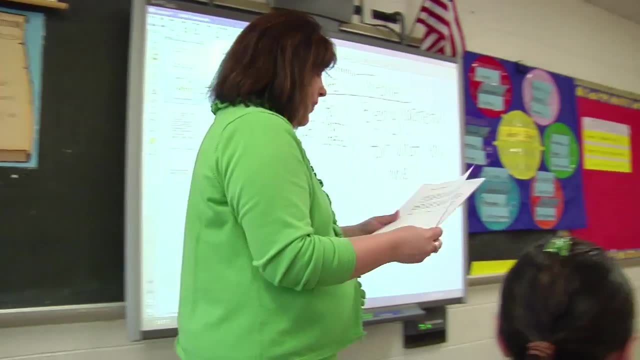 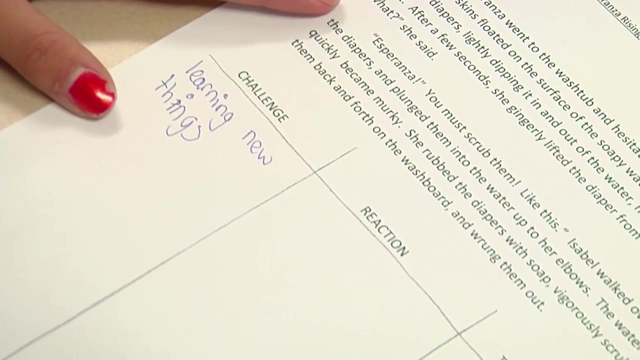 to read it, write down what the challenge is, how esperanza reacts and the possible theme. okay, as soon as you get a paper, you can work on this. okay, what was esperanza's reaction? for the way she was? she had to learn how to scrub a diaper. it was probably like weird, because she she doesn't. 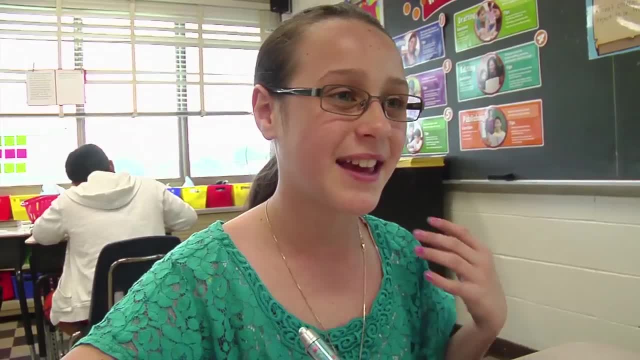 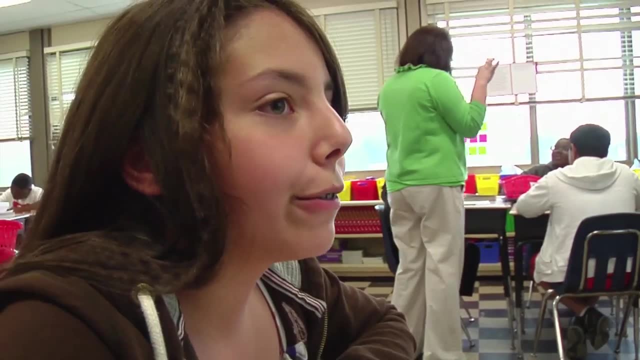 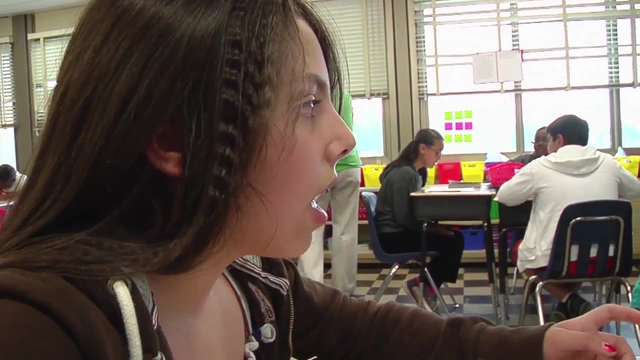 usually do that at where she lives, because usually servants do it for her. yeah, so she was just learning. what do you guys think the theme is of that? this what we talked about, how she was cringed and she's learning new things. um, no matter, like how you think how gross it is and how thing how it, how. 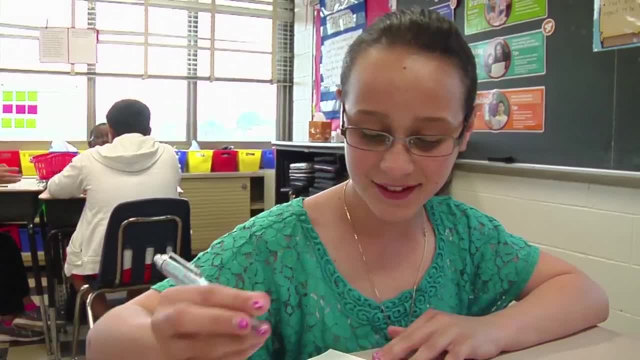 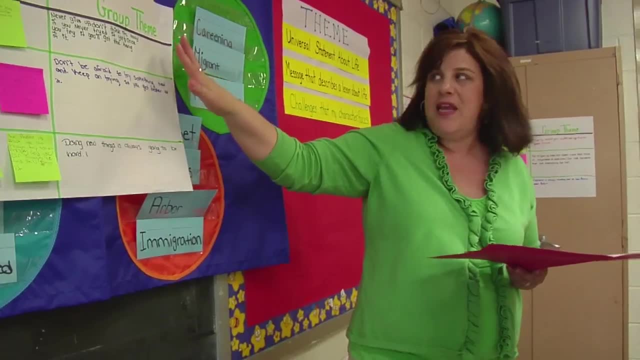 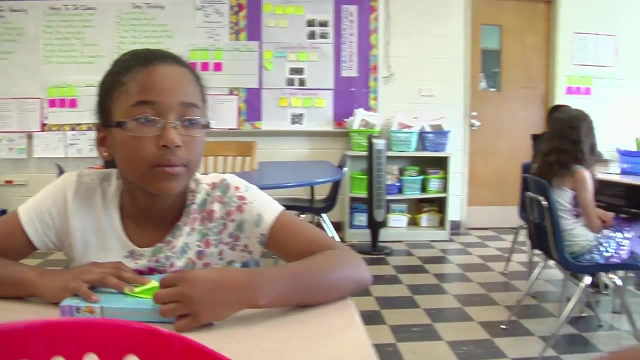 tough it is, you should always try to do it. so i will continue to use the esperanza chapter book to help them understand how to scrub a diaper, understand theme and see how the different characters play out and, by the end of the book, truly seeing what the author was trying to teach us. i think the theme is like like it said in the 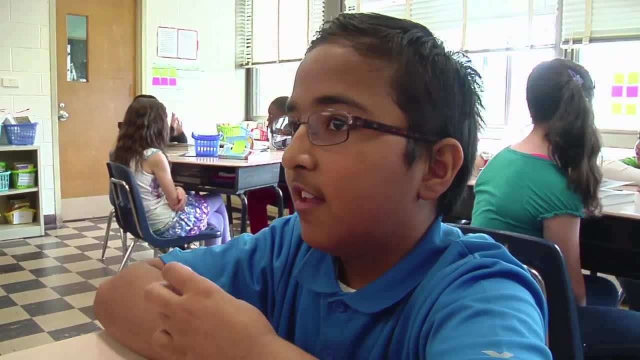 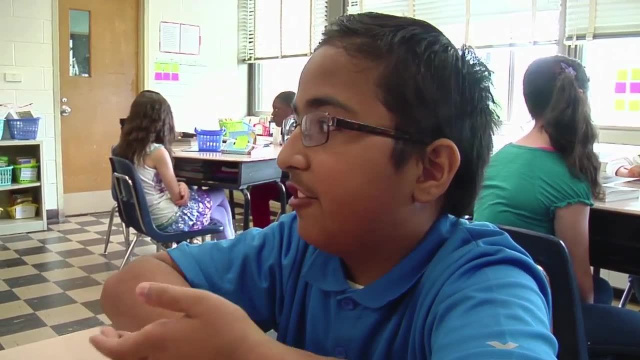 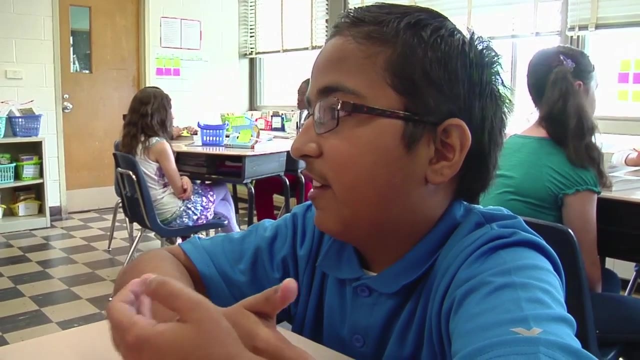 story there's: there is no rose without thorns, like um they're like in life there's always like challenges that you have to face, like when her father died she had to keep on moving. she can't just like stay there and just be upset, because then she can't live her life like good. 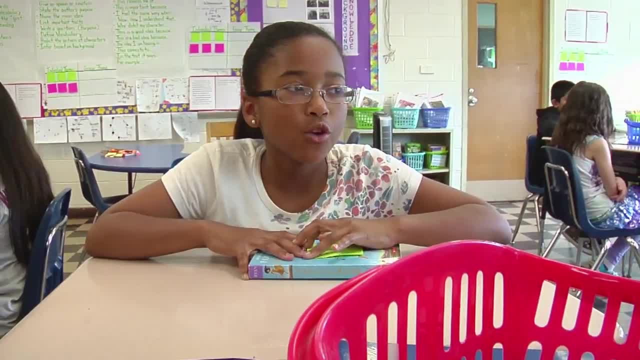 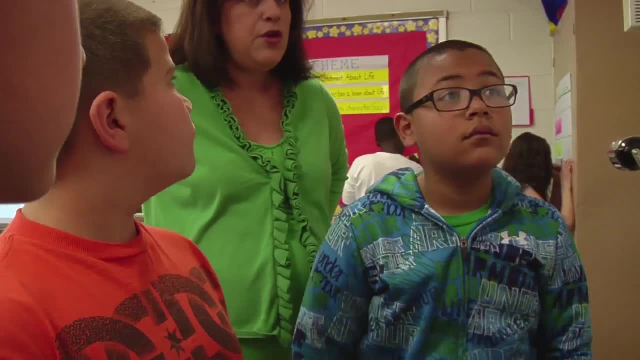 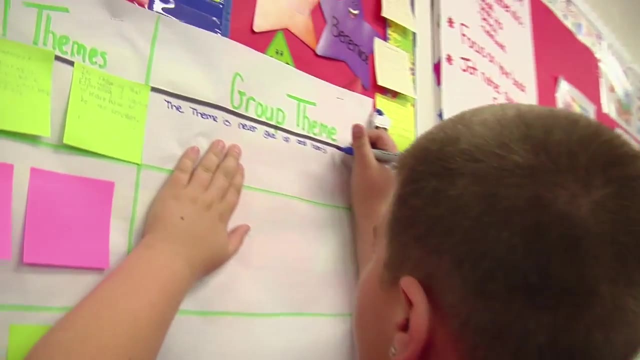 so do you like? you have to move on and stay where your challenge is and succeed it. the carousel activity gives me an opportunity to provide them with many different experiences at one time, so they're not just looking at one piece or looking at a larger text. i'm able to zoom them in on. 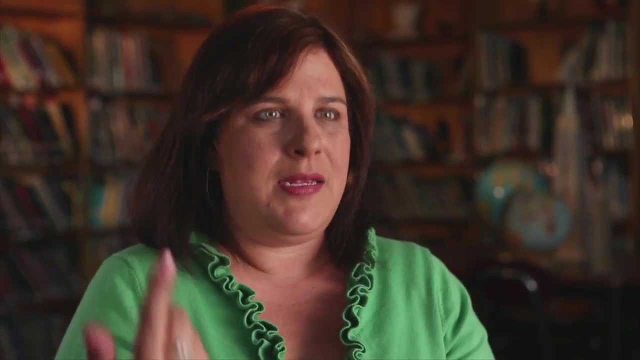 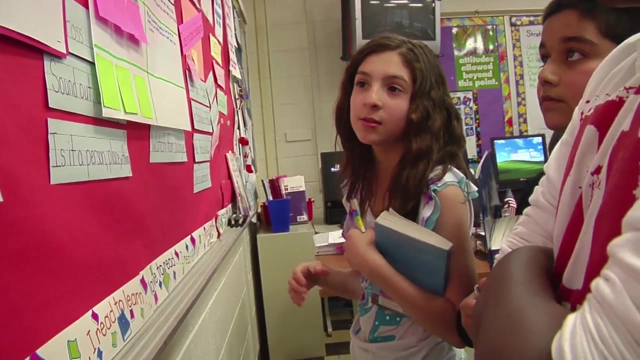 something specific and then move them to something else specific so they can make some connections. i think her mom was rich before and they had money, so she didn't have to wear her hair down like we should. not, she wasn't working and like the thing i just noticed that we all 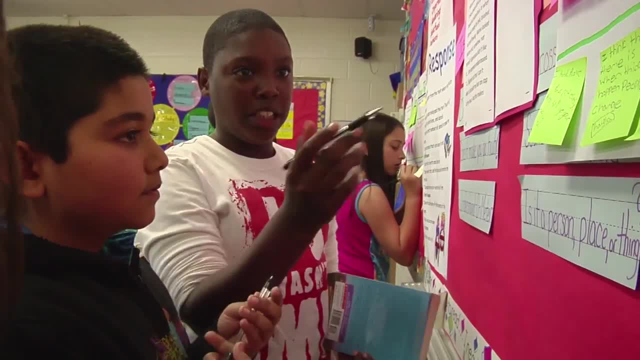 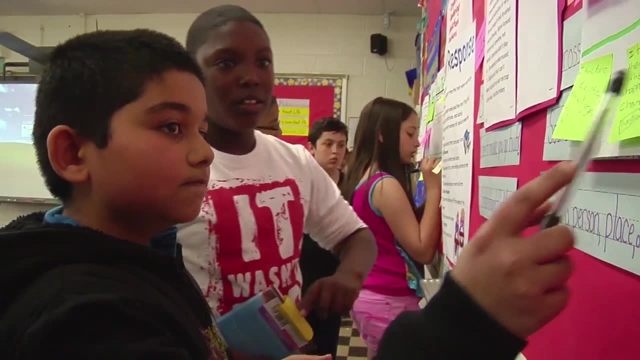 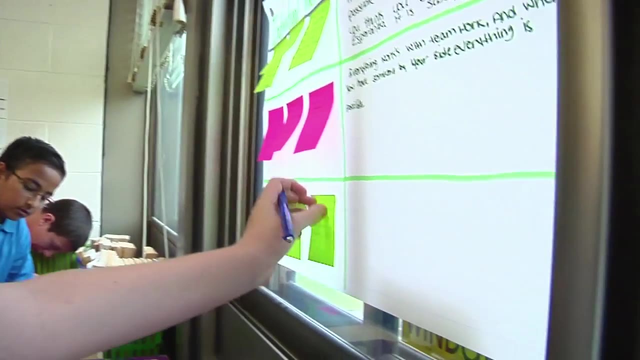 we all like we had like the thing in our head like was changed. yeah, because, like i had it in my head but i didn't want to put it again- always have a friend to help you with something that you need help with, okay, so it's what's talking about. it's all about getting help, yeah, and 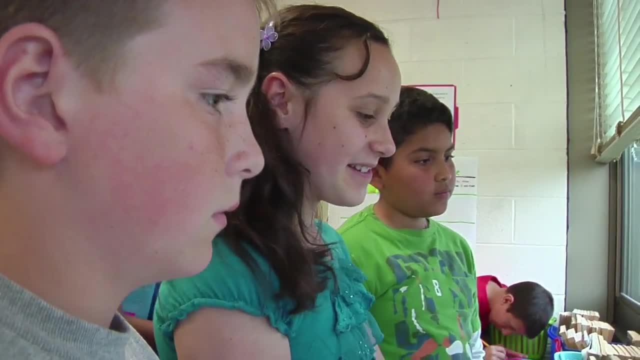 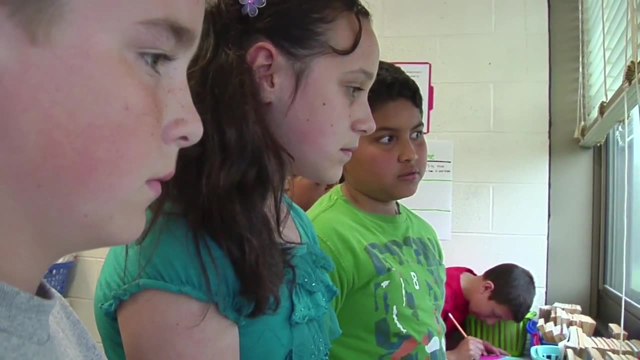 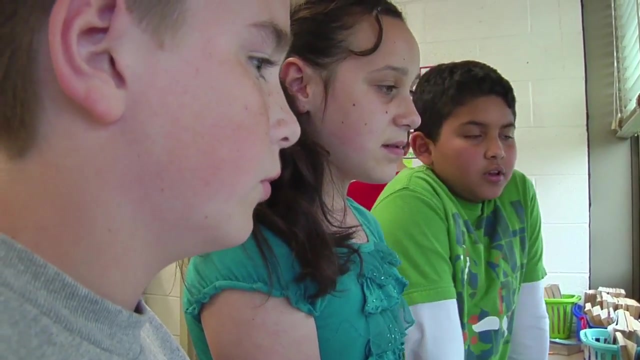 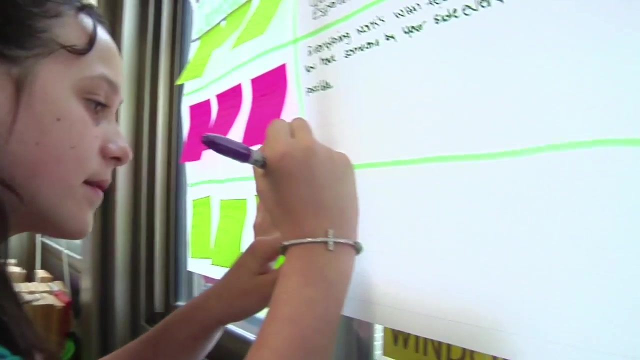 learn that you can learn something new by someone teaching, teaching you it. so the theme is always: well, not okay, go get help. yeah, like you, you can always have someone to help you if you can learn something new every day by someone helping. these are the group themes that you came up with that she shouldn't give up.